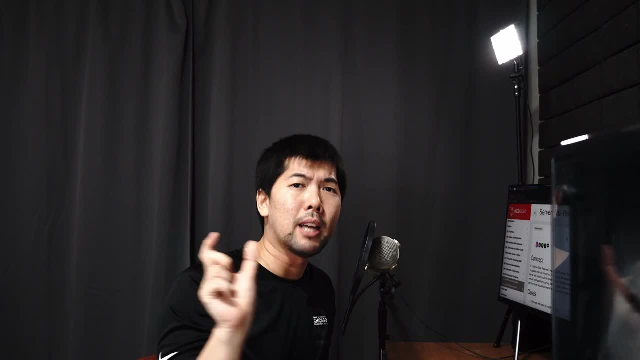 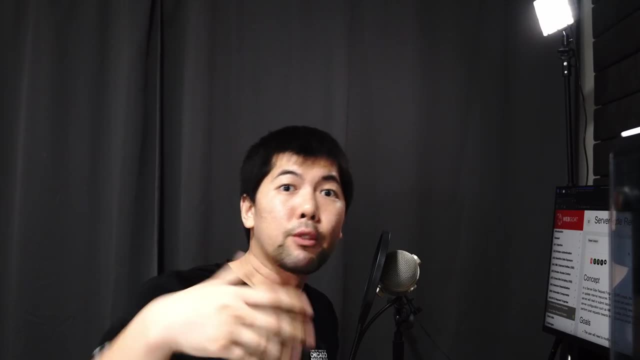 would send you a malicious link And the link would contain, for example, bankcom, followed by the action of withdrawal of money, And once you clicked onto it, because you already logged in, you would transfer money out of your account, doing and running actions on your behalf. 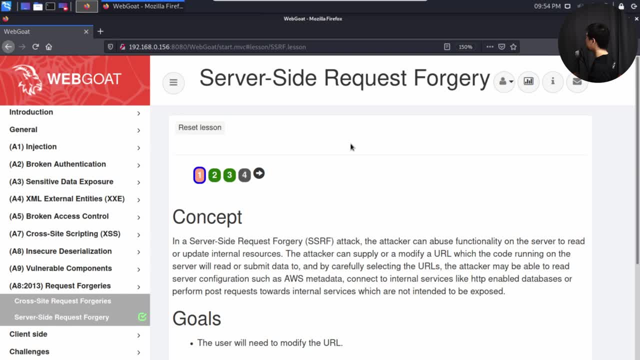 So in this case we have server-side request forgery. So we have here WebCode, which is a vulnerable web application system for us to run all our ethical hacking techniques on, And in this case we have server-side request forgery. So once again, I know you encounter a lot of technical 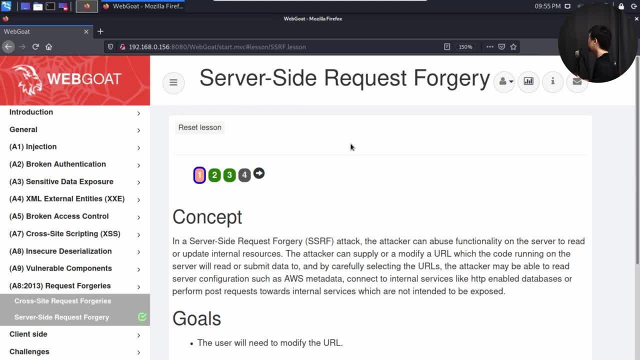 terms in the world of ethical hacking and penetration testing. but no worries, we will learn it. We'll break it down easily and simply so that we understand it fully. So here, server-side means that in the state of previously, where we are sending it over to the user. 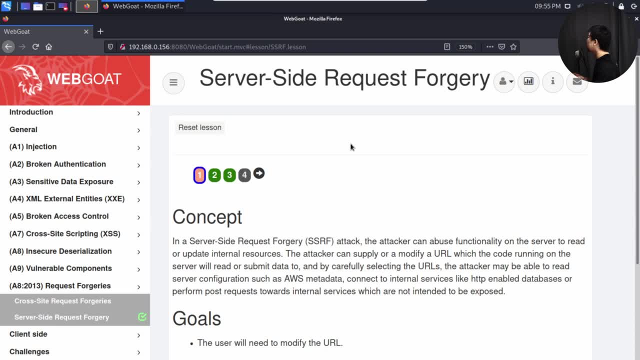 in this case, we're taking advantage of the server, who may have already been authenticated to other services, other resources, And as a result of that, we can make advantage of the server-side authentication to launch those request forgery on behalf of the server. So how can we do? 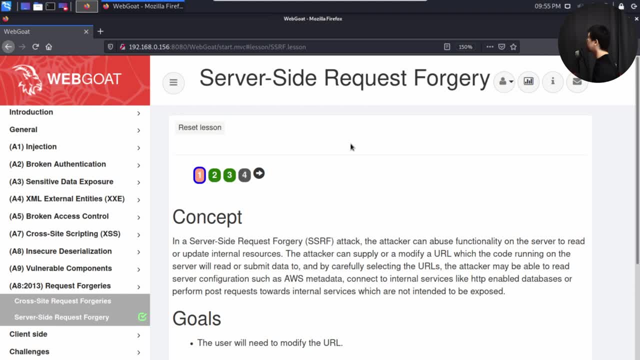 that, And this comes in several ways of thinking, several ways of attacking the server. So the first thing is to think about what kind of possibly services that the server could be subscribed to and, as you can see here, there are certain internal services like an internal database system, an. 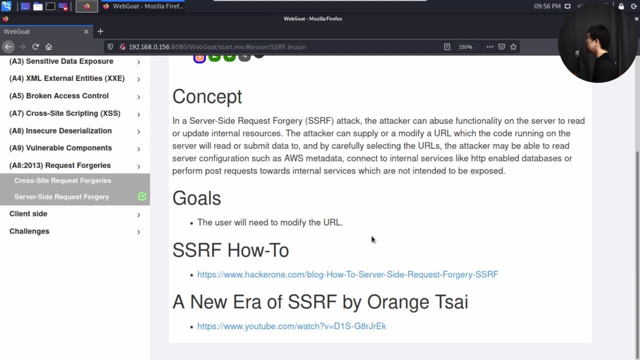 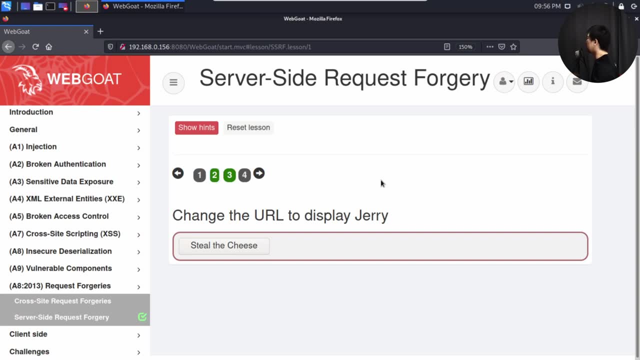 internal HTTP server and so on and so forth, or even internal storage system that you can access into. So, of course, over here we have a very simple lab that we can actually run a lesson on. So once you click on the following, it states the following here: change the URL to display. 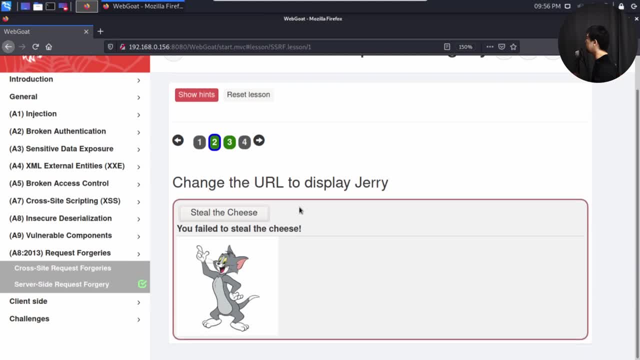 Jerry. So once I click on steal the cheese and it states the following: you failed to steal the cheese, Okay. so what's going on? So let's go ahead and inspect what is happening here. So I can do a right click on the server and I can see that the server is not subscribed to the server. So I can. 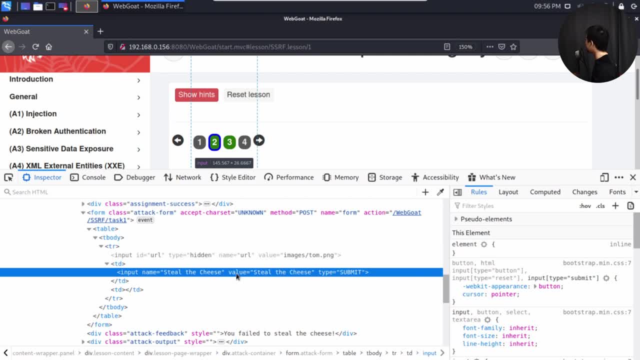 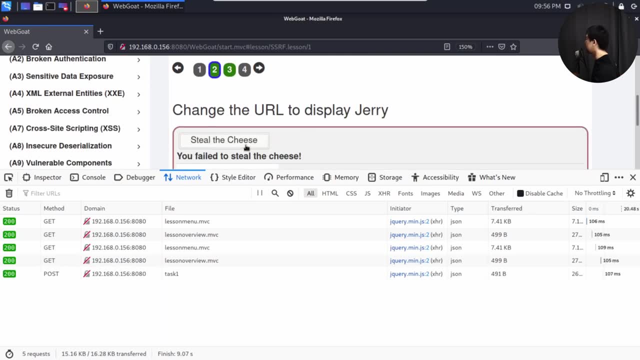 click and click on our inspect element And we can see the following: all right, there's a submission of input name And we can go ahead and click on the network. Okay, so on network, I'll go ahead and click the following: steal the cheese. Okay, so we have done that. I'll pause it right here And this: 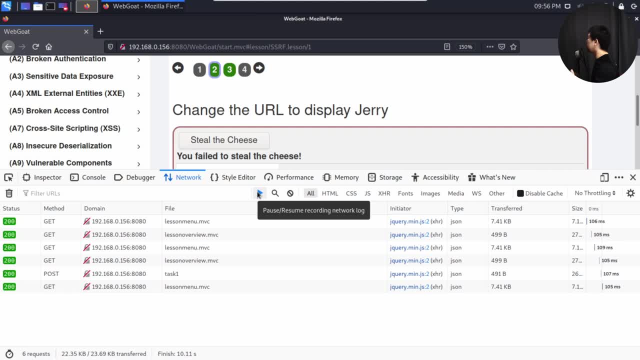 is web developer, And web developer is a very. it's a very useful technology for us to actually launch attacks against different web services and try to see how they're responding to different kind of payloads that we're sending over. So we have task one right here, And this is a post method. 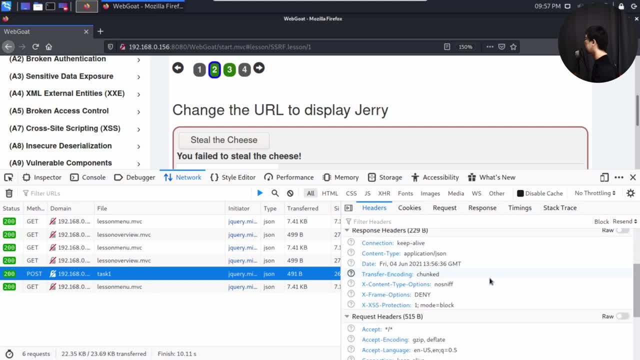 And, of course, as you can see, on the right side, we have the haters. Okay, we can examine the haters, we can examine the request haters, and the list goes on, And we have, of course, the request. 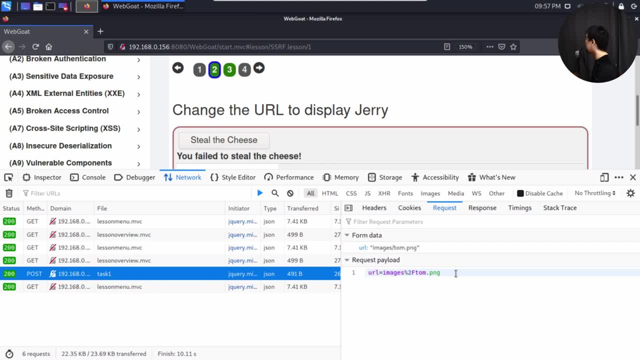 here And this is the request payload. So we have images tompng And then we got a response right here. Okay states the following feedback: you failed to steal the cheese in the output And of course, attempt was made. true lesson completed is false. So what we can do here is do a right click. 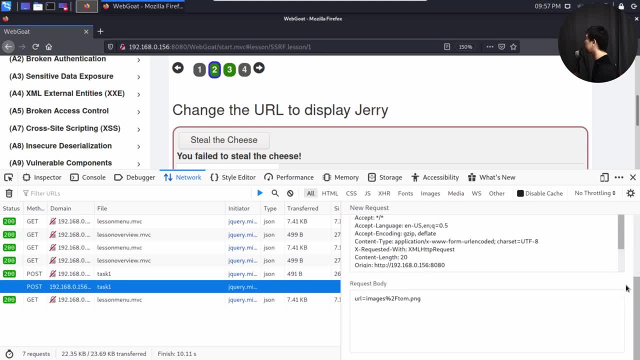 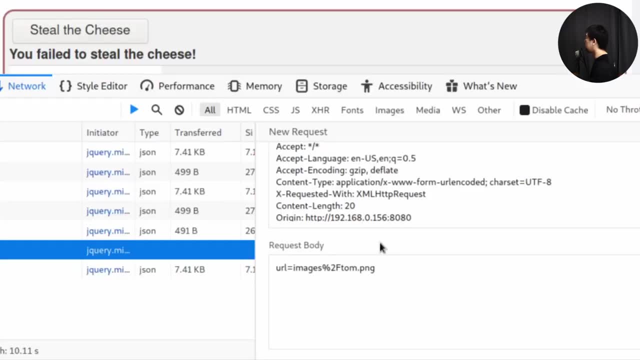 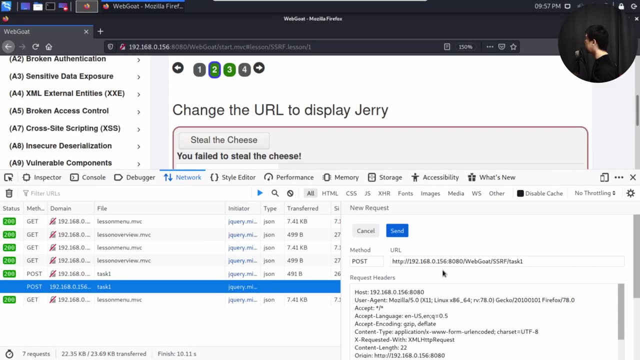 and click edit and resend. Okay, so in this case, if I scroll down further, we can see here is to change the following, which is the request body, And we'll change this from Tom. I can backspace and I can change this to Jerry And let's go ahead and send it over into. 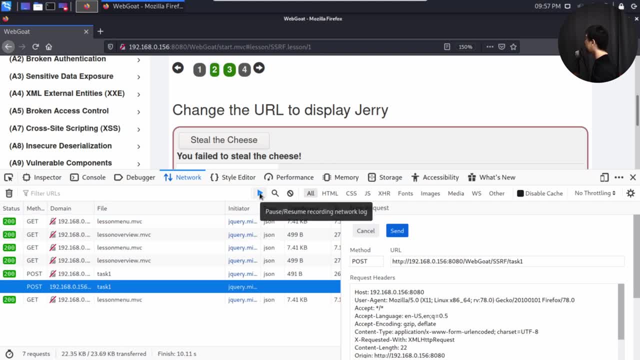 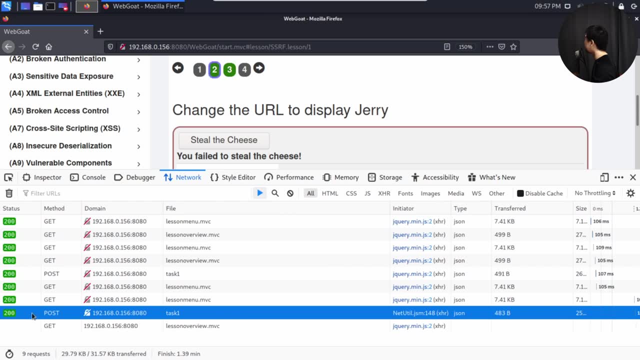 the site and see what happens here. Okay, I'll go ahead and resume recording network lock And I'll go ahead and click send Right done. So we go back over here on the post 200.. So we got a status 200,. 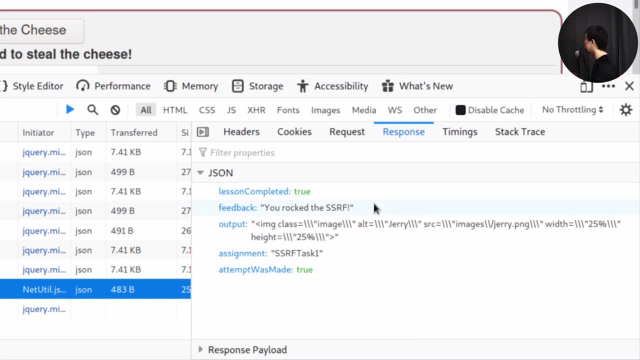 clicked on it And we can see right here: lesson completed. you rocked the server website request forgery. And right here we can see the following source images: jerrypng and temp was made. That's it. as quickly as that we manage to see and view the jerrypng, All right. 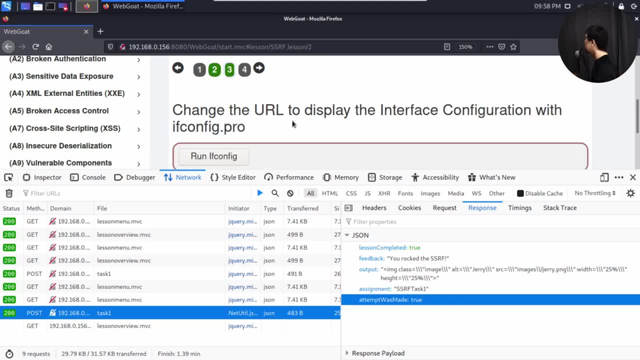 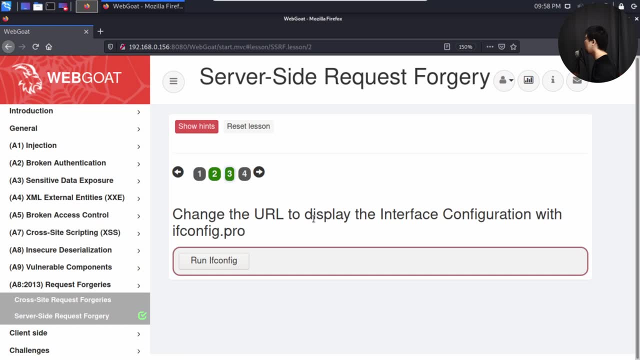 so, moving on into the next session, all right, we have the following: change the URL to display the interface configuration with ifconfigpro. So if you go to ifconfigpro, you'll be able to see your IP address, able to see all the information about where you're assessing from. All right, so if I 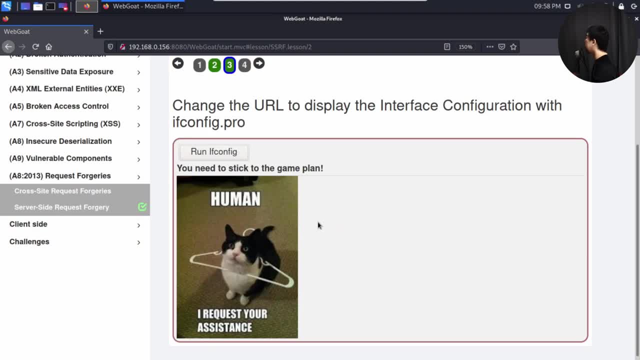 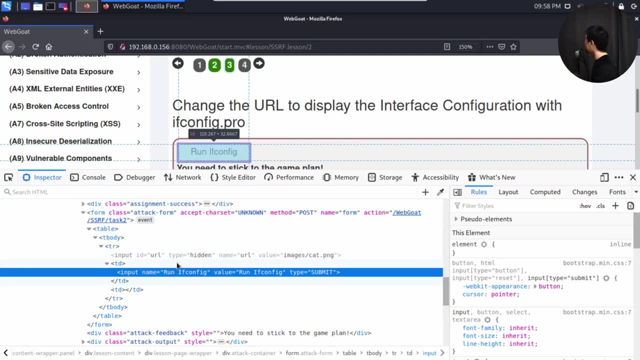 clicked on it. now you'll see the following: you need To stick to the game plan. So what else can we do now? Okay, so once again, do a right click. All right, you can do an inspect element And we can see here there is a particular form, class, all. 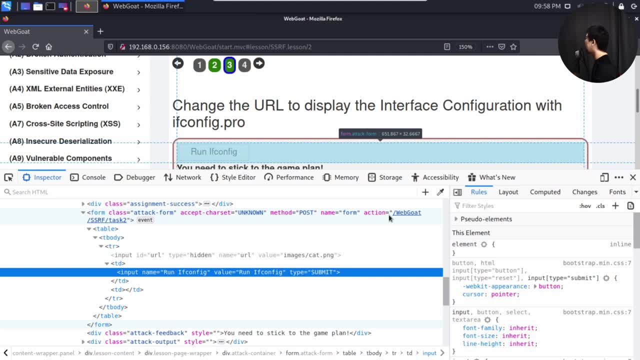 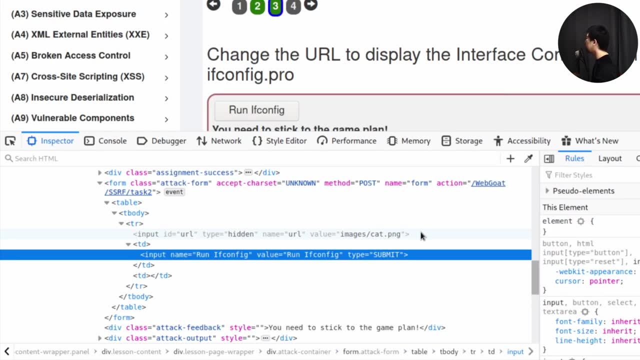 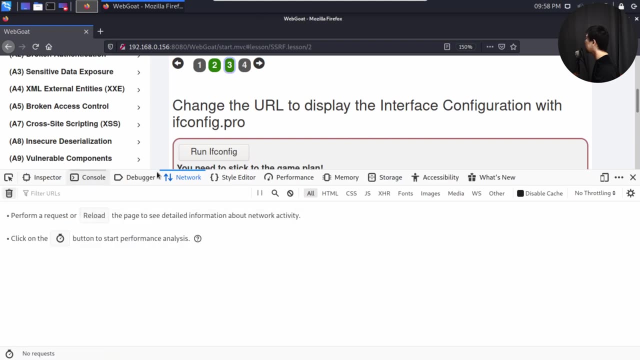 right attack form: accept chart set method form action. And we have here a hidden field. All right, in this case, input ID, URL type, hidden name, URL value, images: slash cat dot PNG. So what can we do here is to go back to the network web developer tab. okay, I can go and clear this one And I can. 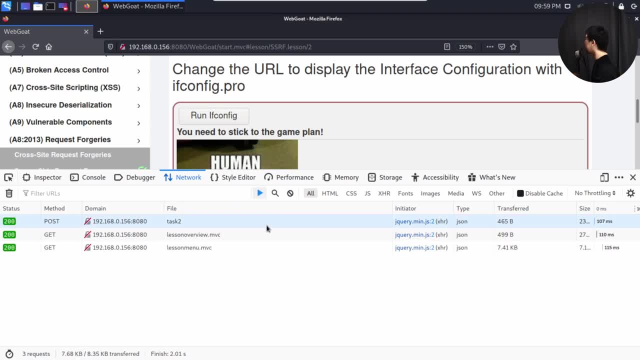 see the following: run ifconfig right now And I'll pause it right here. Okay, so I can click under the post task two: All right, and we can see. here we have the requests And likewise in this case we have images- cat dot, PNG. So let's go ahead and change this and see what happens. All 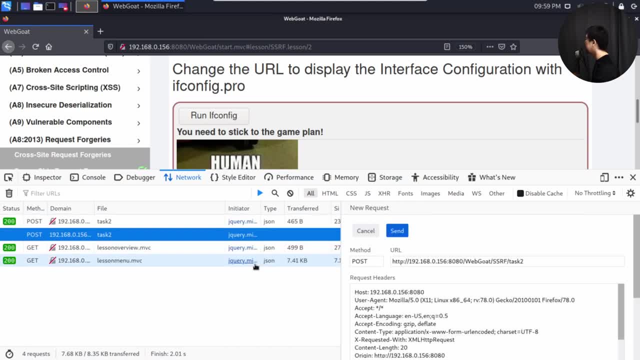 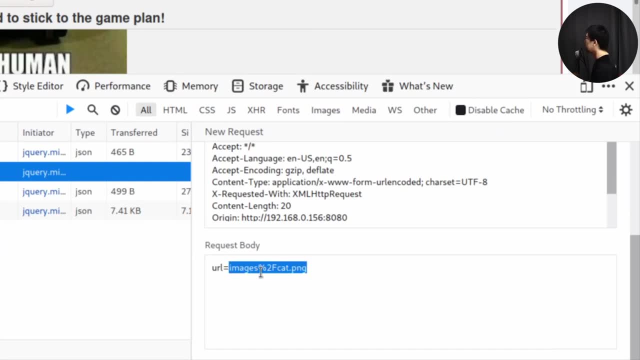 right, so do a right click on task two: edit and resend. Okay, and I'll scroll all the way down. And now I will change the URL. In this case, I'll change it to the target or in this case it will. 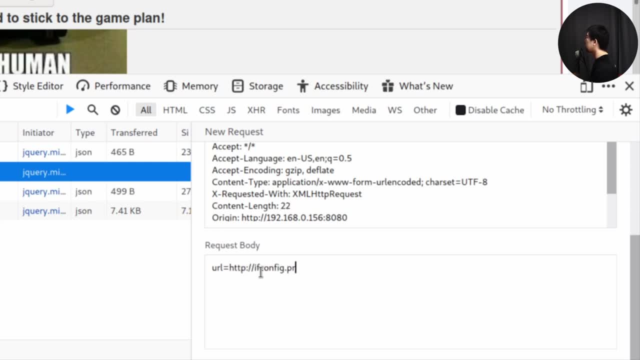 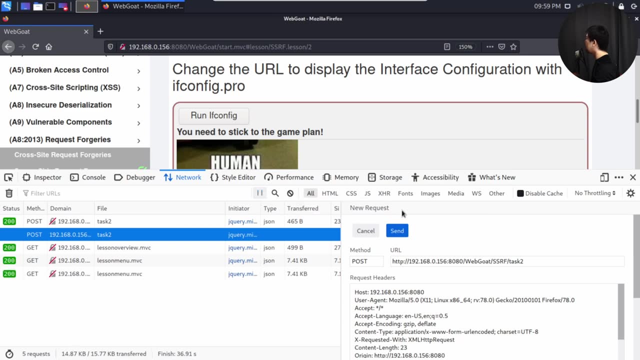 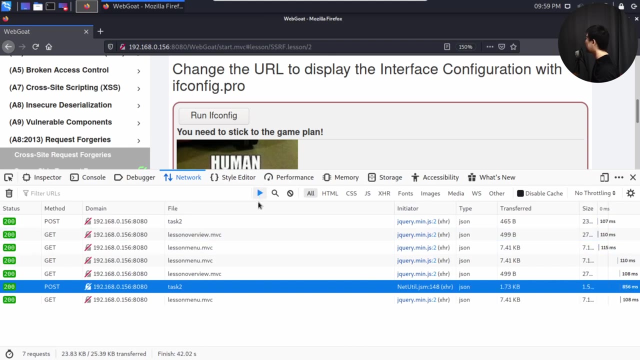 be HTTP, followed by slash, slash, ifconfig, dot P. R. O. Okay, so that's it, And all you got to do now is to play or resume the recording of the network log And in three, two, one, we'll click send. Okay, and that's it. We're done So. 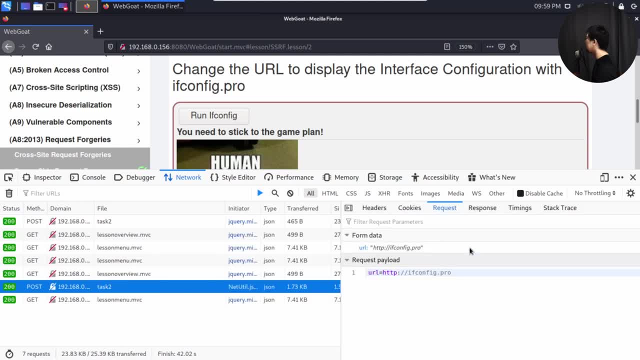 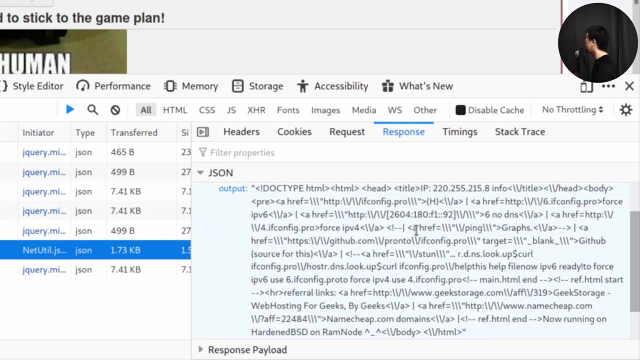 let's go ahead and take a look at the post. So this is the status 200. clicked on it And we can see in a response you rocked the server sign request forgery. scroll down a little further and you can actually see all the information over here. So we have ifconfig. All right, we have the. 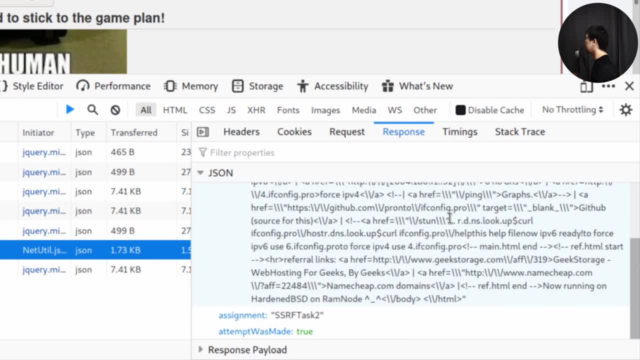 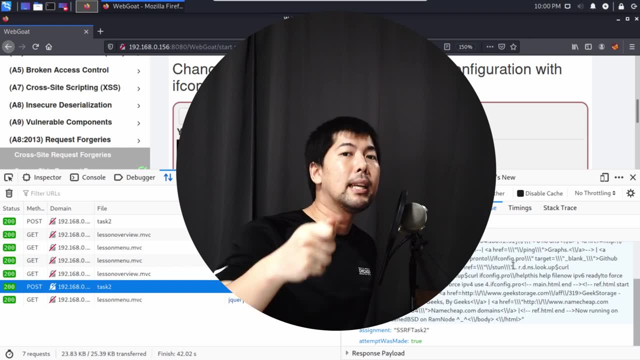 task. we have information about domains and all these different details about the user. So, as you have seen here, what's happening is that because the website is actually posting over- okay, into another site, so it could be a resource, internal resource- that the web application server has. 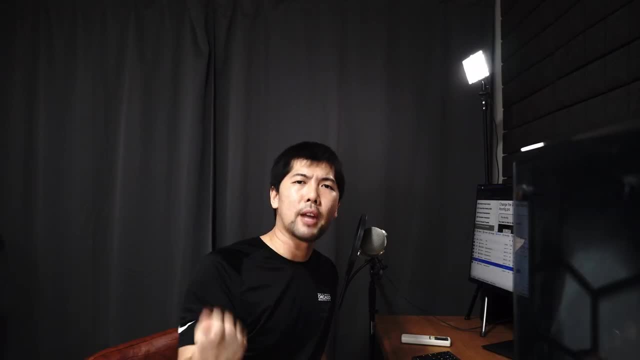 this is called server sign request forgery because the whole idea is that the service authenticated specific resource service And once you were able to make the website actually go over these resources out as they are authenticated, they will do those actions as a result of the 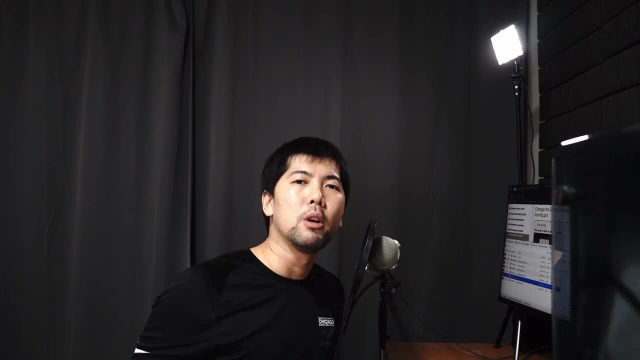 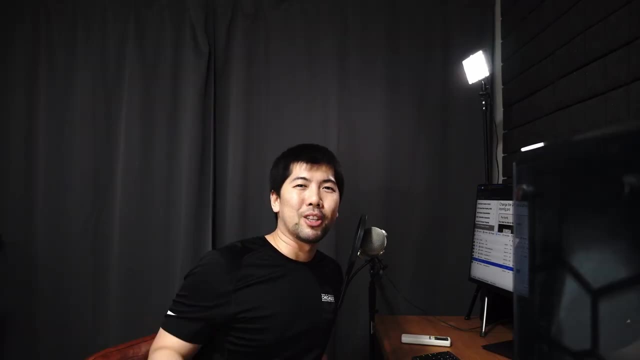 hacking attempt. So, once again, I hope you'll learn something valuable in today's tutorial and will like share, subscribe and turn on notification so that you can be kept abreast of the latest cybersecurity tutorial. Thank you so much, once again, for watching.